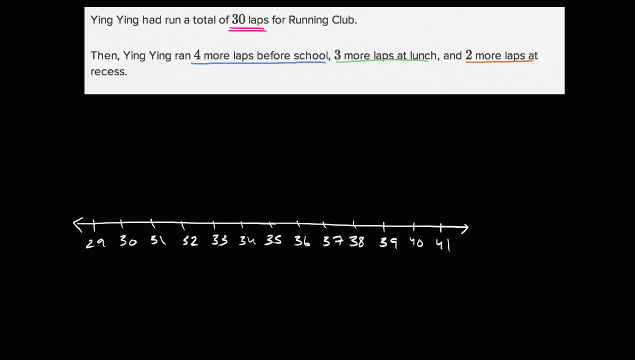 So let's see: Yingying started at 30 laps. So she started at 30 laps for a running club. Then she ran. Yingying ran four more laps before school. So on the number line, if I go four more, 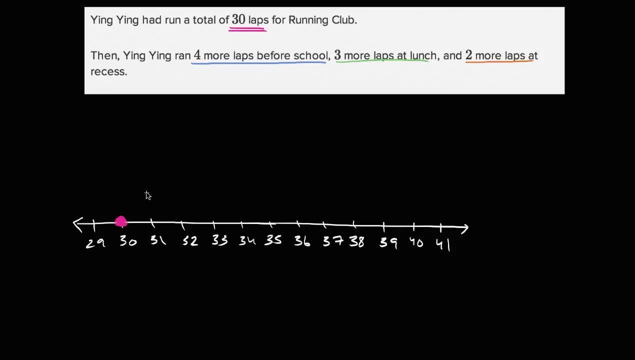 that's going to be to the right. I'm going to be increasing by four. So I'm going to be increasing by one, two, three, four. So those four laps before school take us from 30 to 34.. 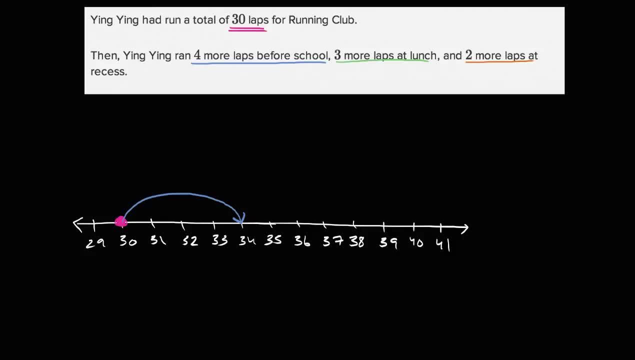 Then she runs three more laps at lunch. So then from 34, she's going to go one, two, three to 37. She's going to go to 37. So that's what those three more laps at lunch do for us. 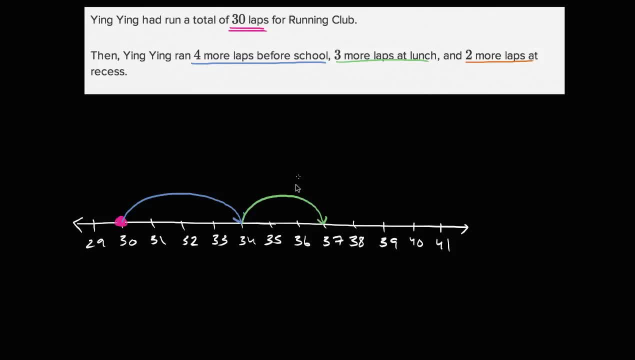 and then two more laps at recess. So she was at 37, and now we're going to go one two to 39. So how many total laps does Yingying run? Well, Yingying runs a total of 39 laps. 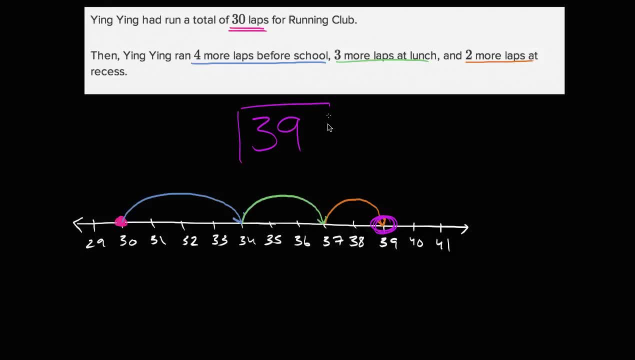 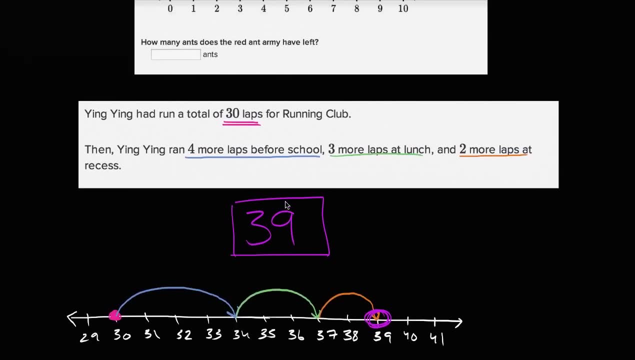 39 laps, and we were able to figure it out using this number line. Now let's do an exercise very similar to this that you might see on Khan Academy. So this one right over here. Actually, let me get rid of the stuff about Yingying. 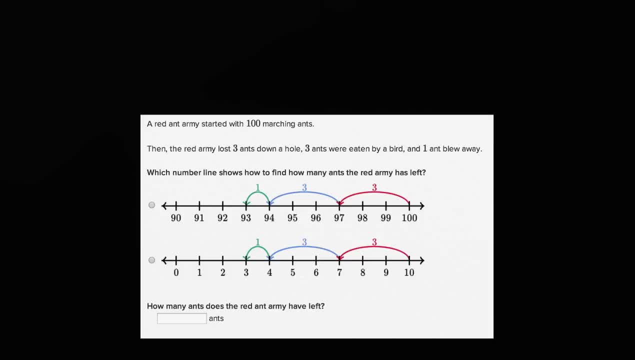 so we don't get confused. So this says- and it's a little bit smaller, but hopefully you can see what it says- A red ant army started with 100 marching ants, So we're going to start with 100, and actually, 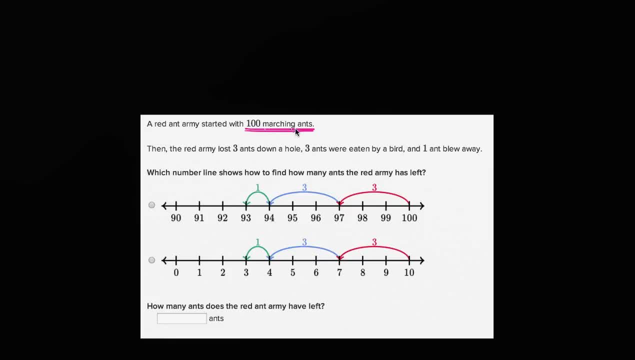 they tell us. well, let me just read the whole thing. It started with 100 marching ants, Then the red army lost three ants down a hole. So actually let me get it. So: lost three ants down a hole. 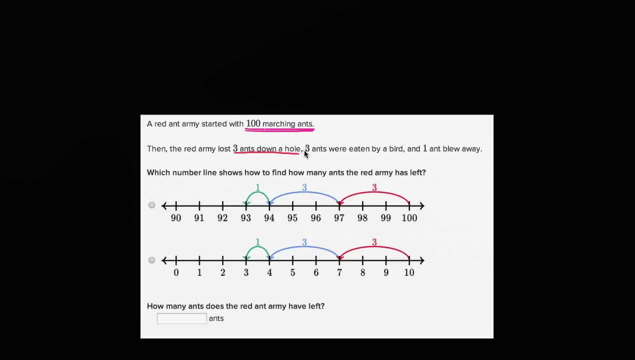 Three ants were eaten by a bird- That's unfortunate- And one ant just blew away. I guess ants are fairly light creatures, so that makes sense. One ant blew away. Which number line shows how to find how many ants the red army has left? 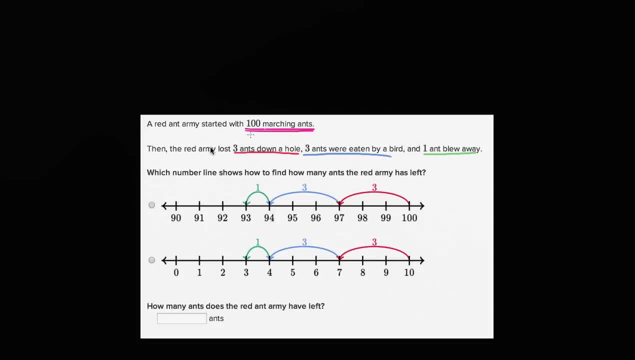 Well, the army started with 100 marching ants. We underlined that over here. So we need to start with 100.. So we need to start with 100.. This one starts with 10.. So I can immediately rule this one out. 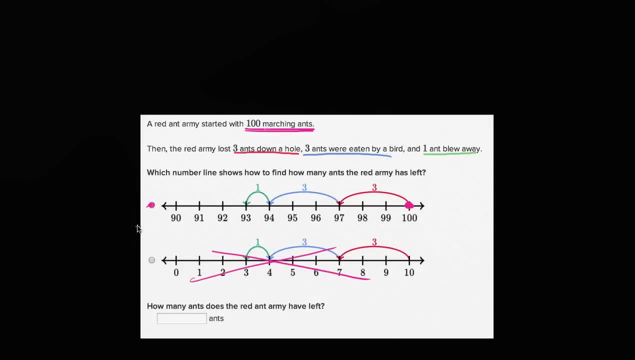 And so we could just select that one. but let's just make sure it makes sense. So we start with 100, and then we lose three ants down a hole. So we're going to go down. Remember, we're losing ants. 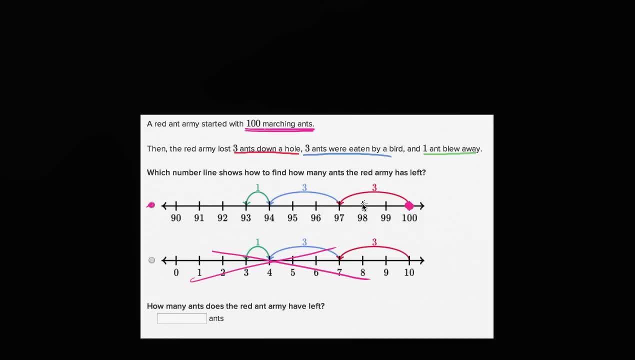 So we're going to go to the left of the number line, We're going to go to lower values, We're going to go down one, two, three. So these are the three ants we lose down a hole. So three down the hole. 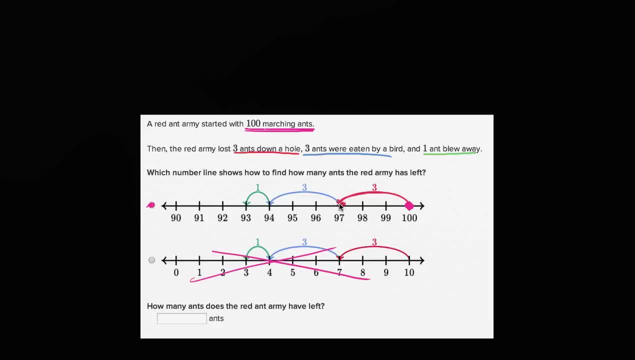 Then we have three that were eaten by a bird, So you're going to lose three more. That's those three right over there. It gets to 94 ants left. And then we have the one ant that gets blown away, So that gets us down to 93 ants left. 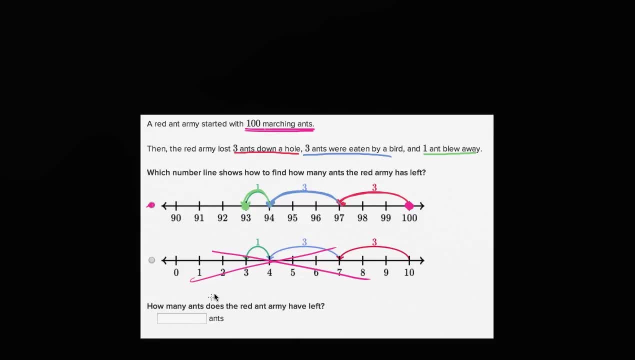 So the red army, or the red ant army, has 93 ants left, 93.. 93 ants left And we are done.